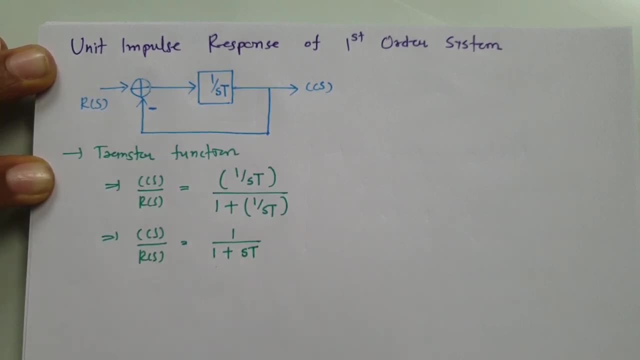 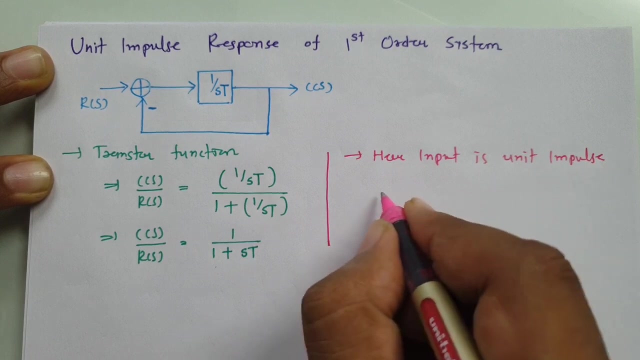 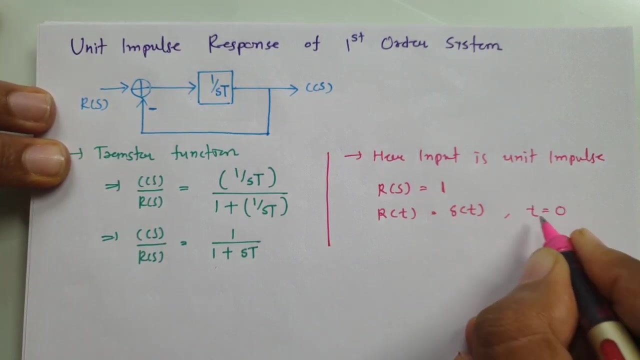 transfer function. Now, in this system our input is unit impulse. So for unit impulse input, R of S, that is equals to 1, and for time domain, R of T, that is del T. So impulse is there at time T is equals to 0. Otherwise its value is 0. for 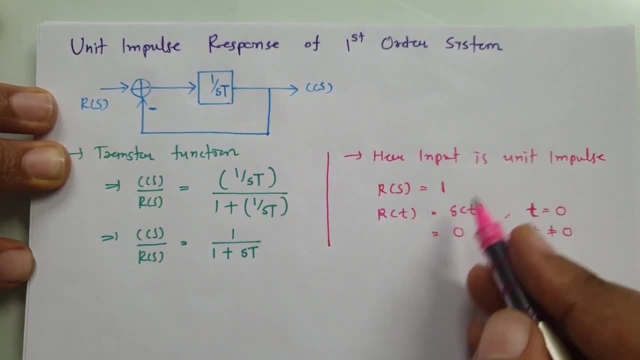 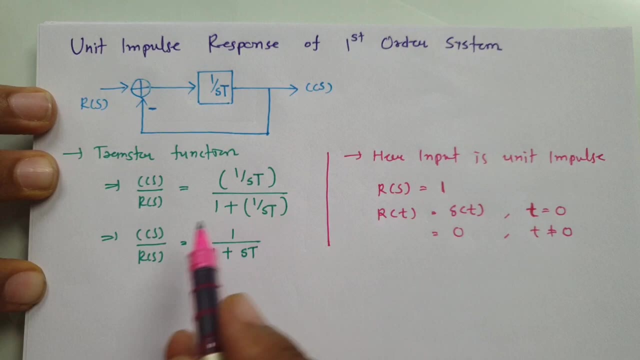 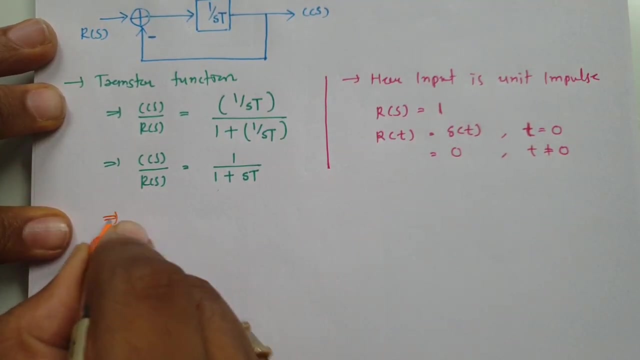 T is not equals to 0.. So that is how impulse signal that is there with us. I'll show you graphically also. So here our agenda is to identify C of S in Laplace domain and in time domain, Right. So here, as per this, transfer function C of S, that is, input R of S, into 1 divided by 1 plus. 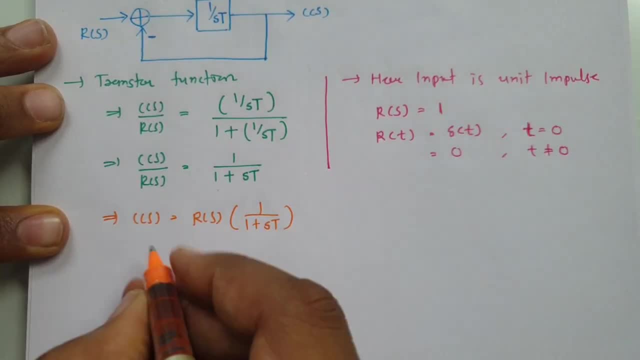 S into T, where this R of S, that is 1.. So we can say C of S, that is 1 divided by 1, plus S into T. Now we wanted to have this output in terms of time domain, So let me readjust this So from: 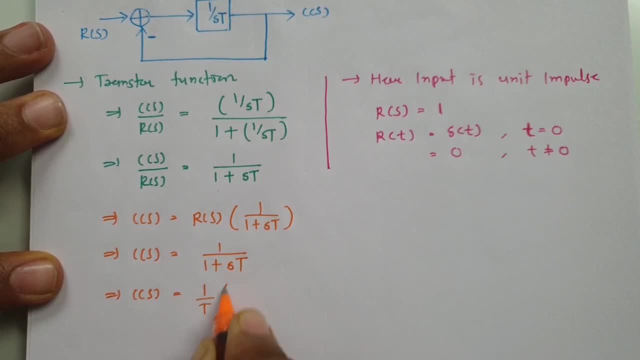 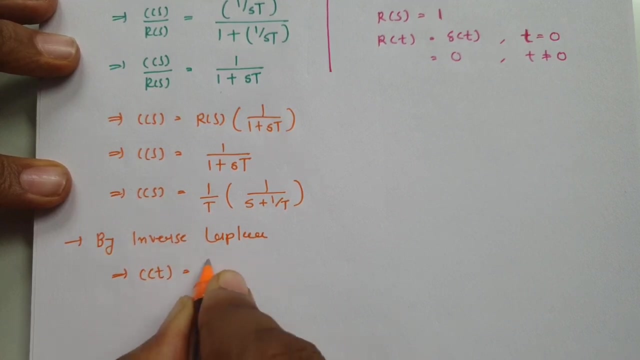 denominator. I'm taking T common, So 1 by T into 1 divided by S plus 1 by capital T. Now to this we can apply inverse, Laplace This output now that will be there in time domain, So 1 by T. 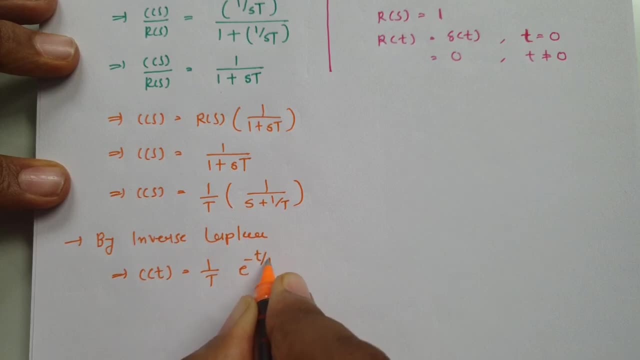 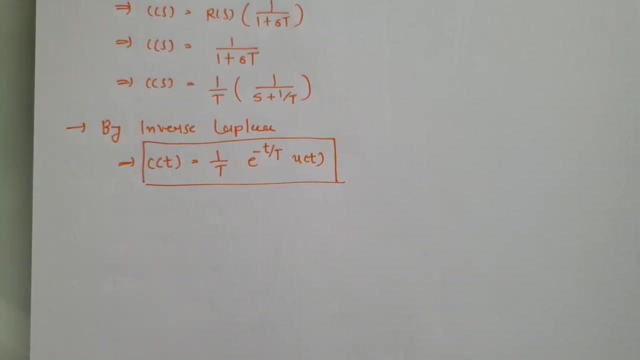 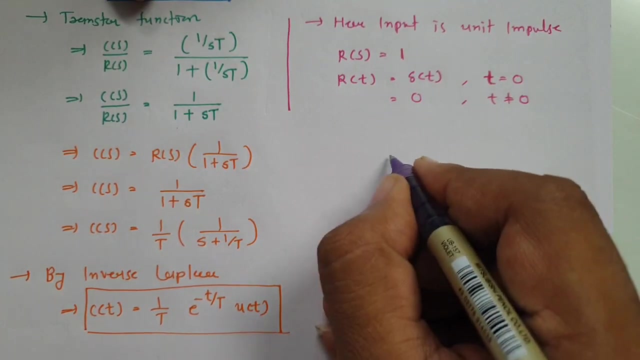 into e to the power minus small t by capital T u of T. So this is how our output C of T will be there in time domain, as if input is impulse. Right Now I'll show you graphically how things are happening. Understand this graphically. Let me plot graphical presentation. So here we have time, Here we have.